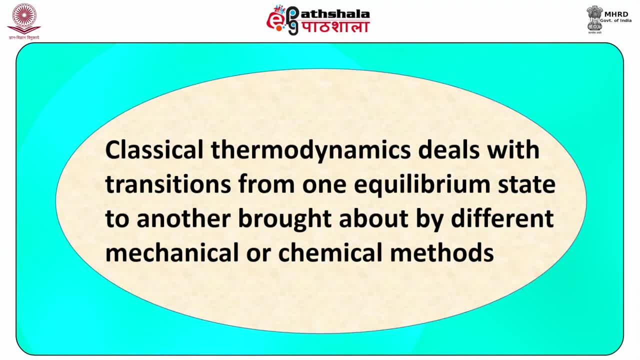 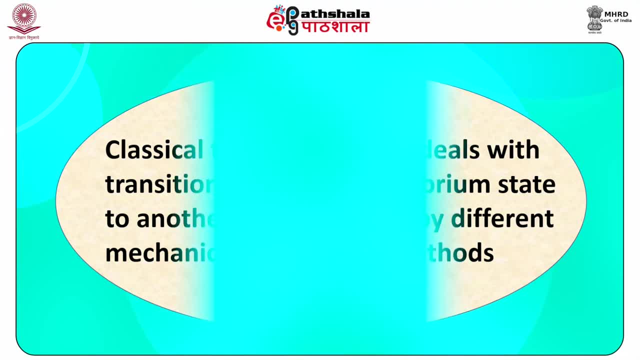 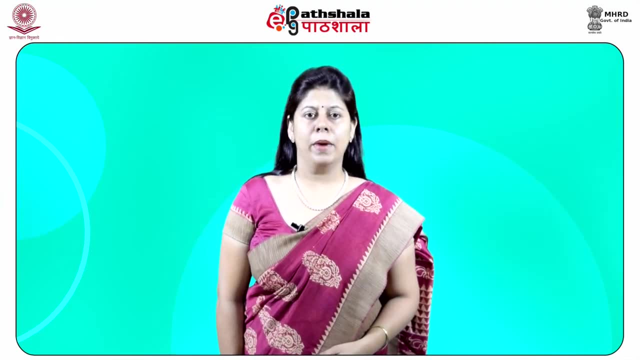 Classical thermodynamics deals with transition from one equilibrium state to another, which brought about by different mechanical or chemical methods. It is not applicable to systems in which transport of heat, charge or matter takes place. Non-equilibrium thermodynamics is that branch of thermodynamics. 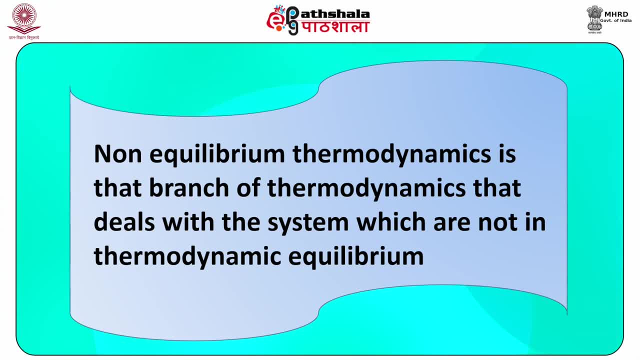 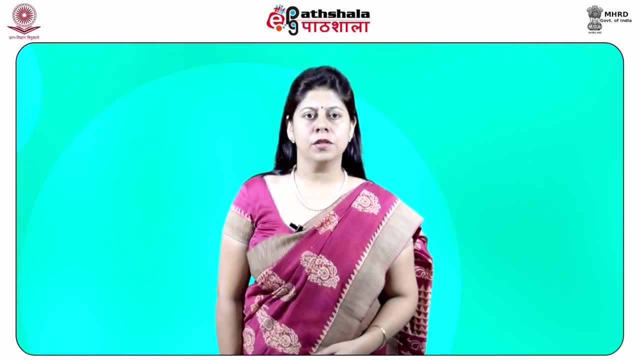 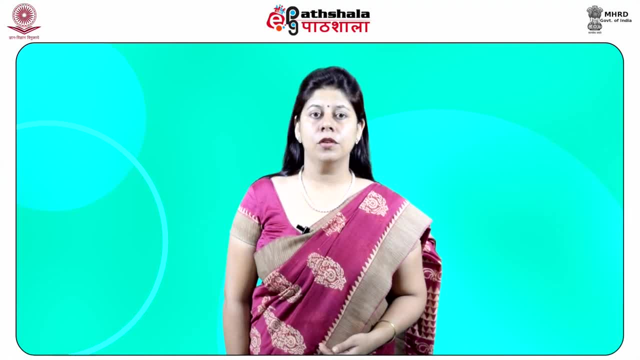 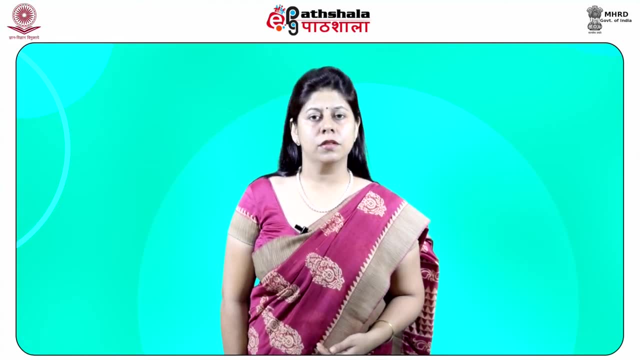 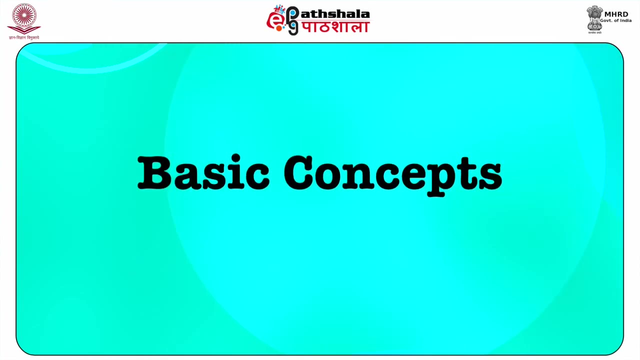 All natural processes occurring are not in thermodynamic equilibrium. Moreover, non-equilibrium state variables should be mathematically related to each other in ways that resemble corresponding relations between equilibrium thermodynamic state variables. Now let us see the basic concepts which you have learnt earlier also. 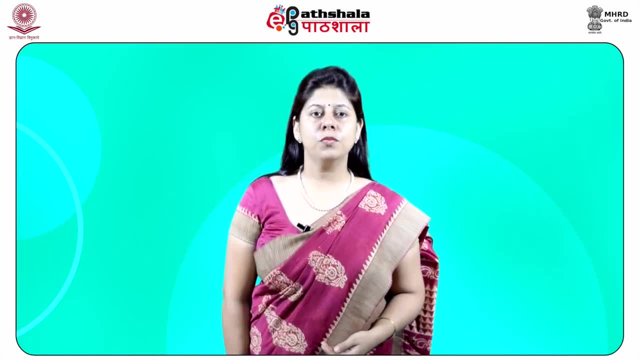 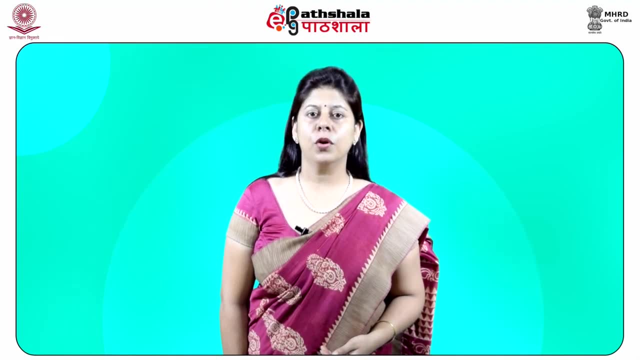 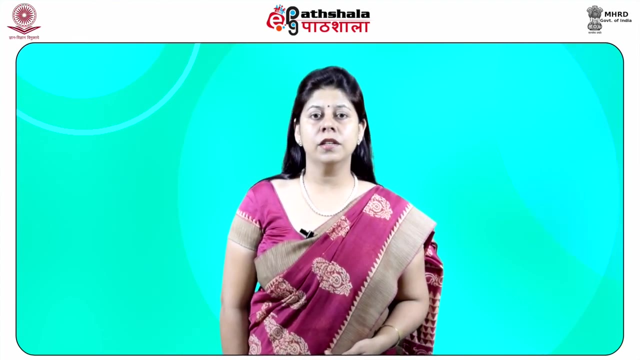 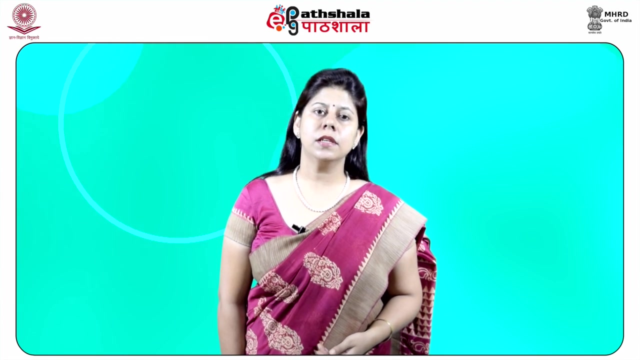 System exhibiting non-equilibrium processes are much more complex than they undergo fluctuation of more extensive quantities. Some boundary conditions which are imposed on them, particularly intensive variables like temperature gradient or distorted collective motions, are called thermodynamic forces. Now discussing different laws of thermodynamics. 0th law of thermodynamics: 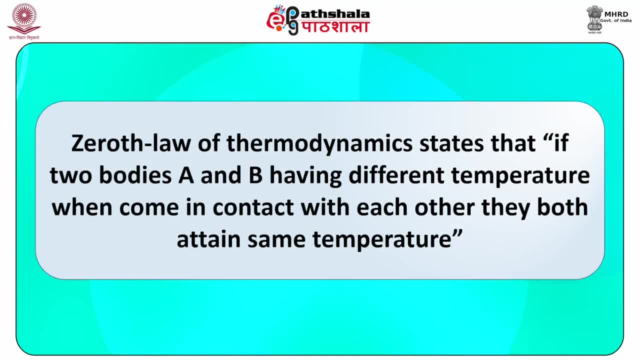 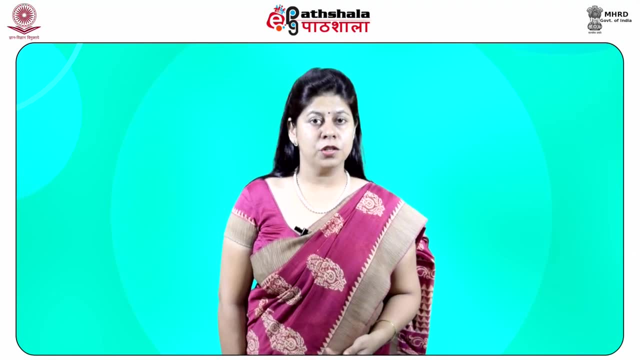 0th law of thermodynamics states that if two bodies, A and B, having different temperature when come in contact with each other, they both attain same temperature. In such system, mass won't get exchanged, but energy is exchanged. Thermometer is based on 0th law. 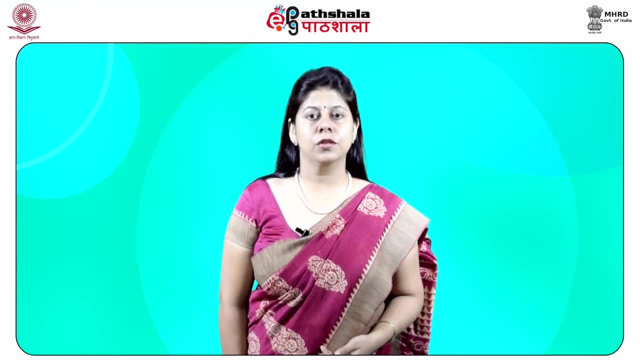 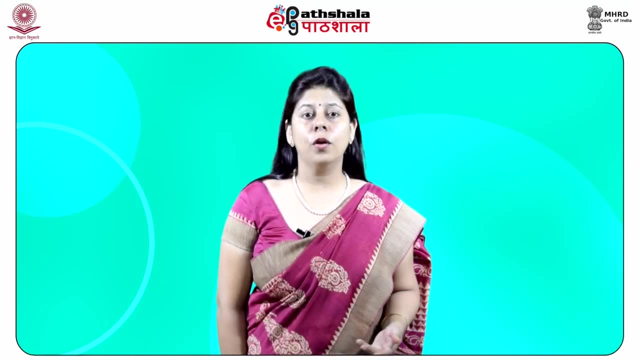 First law of thermodynamics. The first law of thermodynamics is also known as law of conservation of energy, ie energy can neither be created nor be destroyed. This law states that if system absorbs heat from the surrounding- In this case, heat is absorbed from the surrounding- 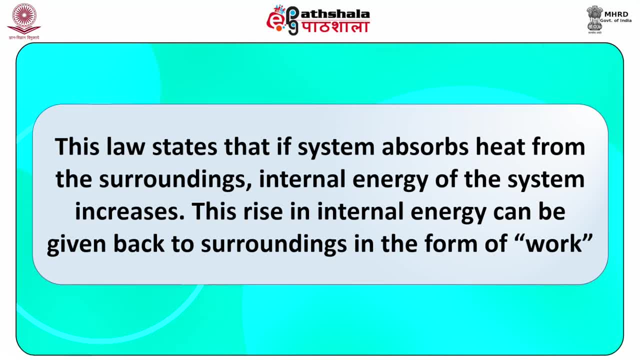 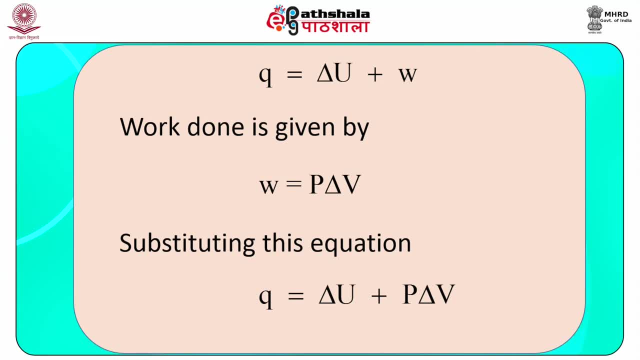 So internal energy of the system increases. This rise in internal energy can be given back to surroundings in the form of work. Mathematical form of the first law is: q is equal to Delta u plus third t. Delta u is direction ie, c. u is direction to moment where delta. 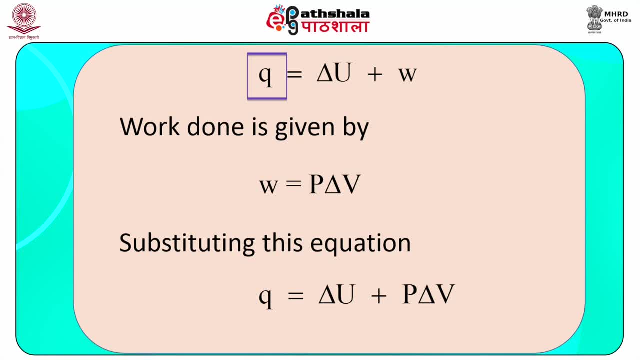 u is change in internal energy, q is gotten as heat absorbed and w is the work done. Delta v is a change in internal energy. This is called pc. We also know that it is given kind of as delta v. By this kind of change we can say that for multiple transmissions, the hertz to the 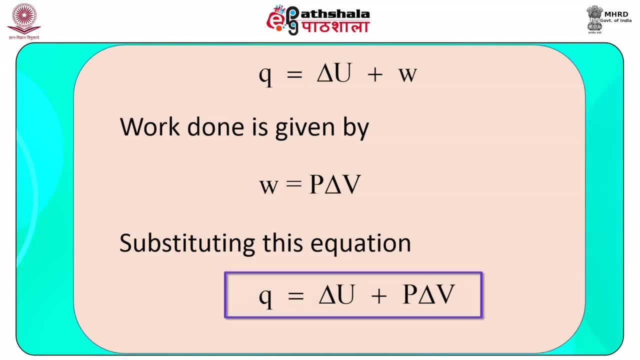 middle of teles meiseen will not die times c into rencontilde. a1is given by rad 1ye and w is a denied dude into delta v. Is it وال? substituting this equation in equation we get: q is equals to delta u plus p, delta v. 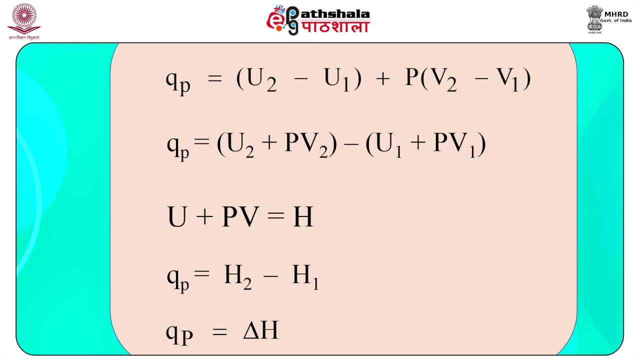 now the heat absorbed. keeping the pressure of system constant will be given by: qp is equals to u2 minus u1 plus p. into the difference of v2 minus v1. or we can write qp as equals to u2 plus pv2 minus u1 plus pv1. in the equation, u denotes the internal energy, p is the pressure. 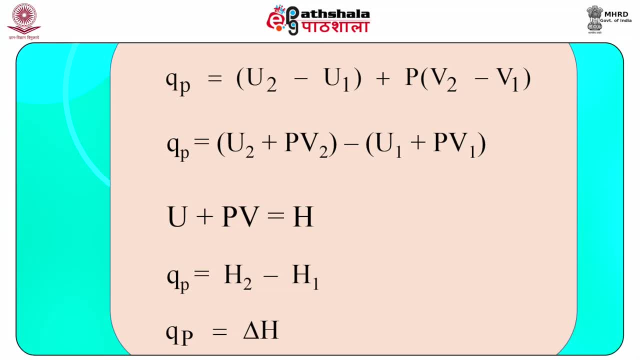 and v is the volume. all three of them are the state functions. therefore, the quantity u plus pv should also be the state function. the quantity u plus pv is equals to h is known as enthalpy, and the change in enthalpy will be related to the volume of the energy which 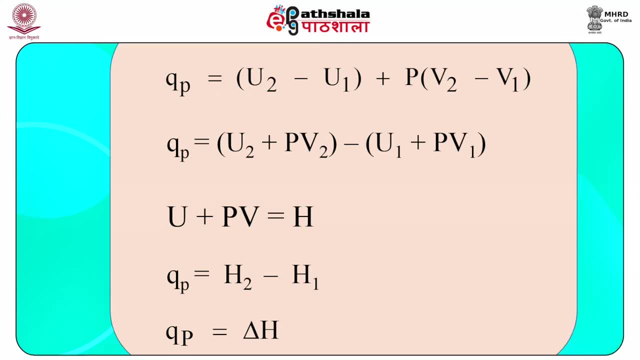 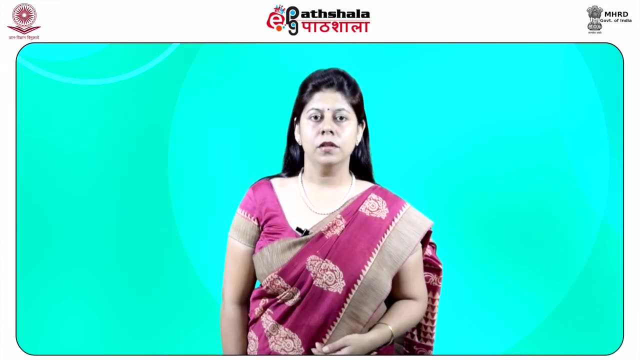 is represented in the equation, we get to the state function u plus pv is known as enthalpy will give amount of heat absorbed at constant pressure. that is, qp is equal to delta h. Now let us see the second law of thermodynamics. The second law of thermodynamics forms the 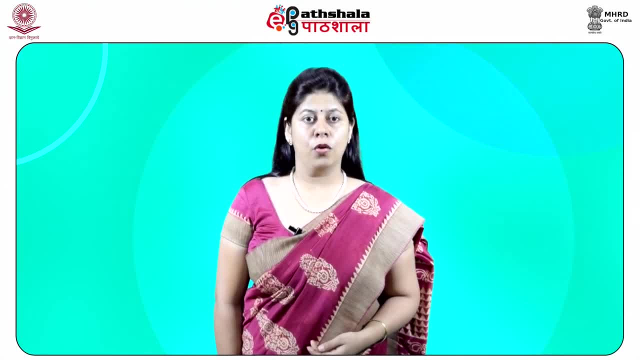 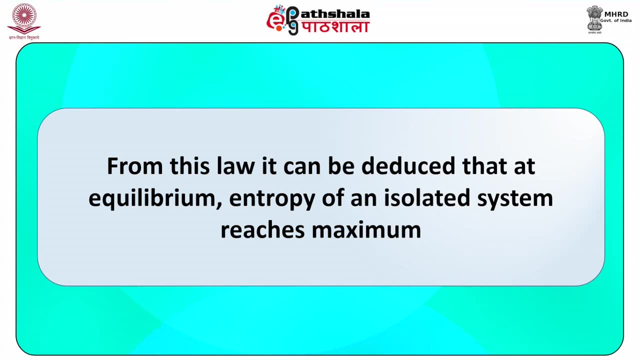 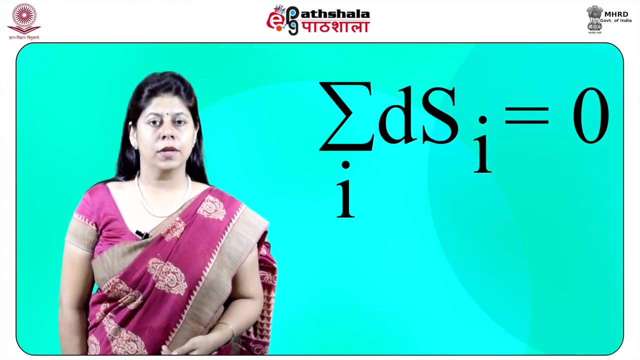 most important law in classical thermodynamics, from which the criteria of spontaneity and equilibrium of a system are derived. From this law it can be deduced that at equilibrium, entropy of an isolated system reaches maximum. At equilibrium, sum of all the components of entropy change is equal to zero. ie summation of ds i is equal to zero. 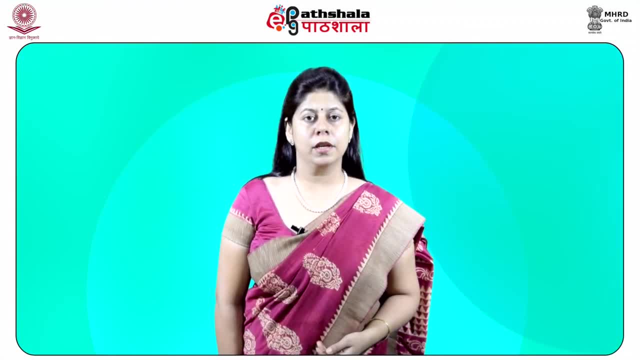 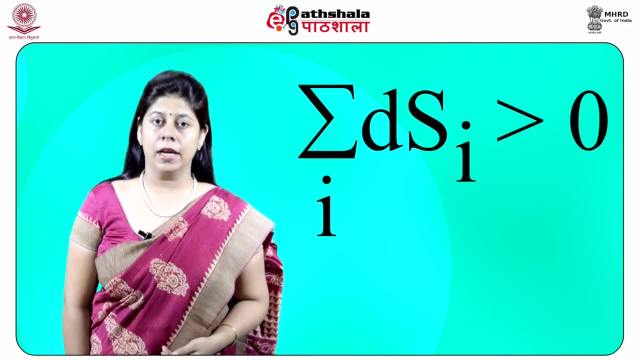 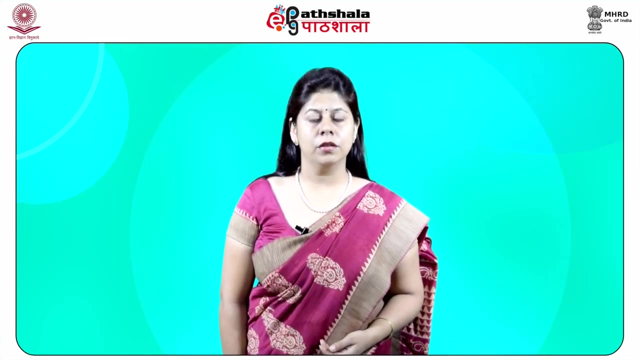 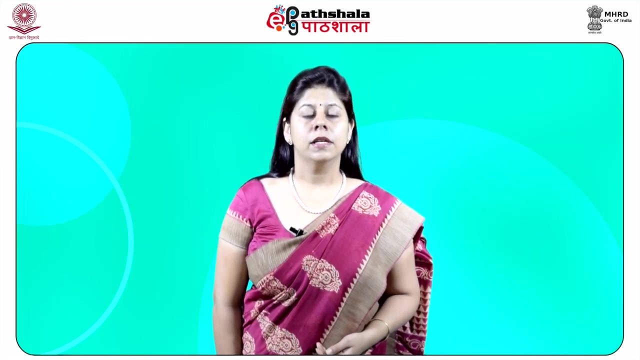 For spontaneous reaction which is moving towards equilibrium state, the sum of all the components of entropy change becomes greater than zero, ie summation of ds i is greater than zero. In the steady state condition, macroscopic properties like pressure composition remain the same with time, but dissipative processes continues to change in a system. 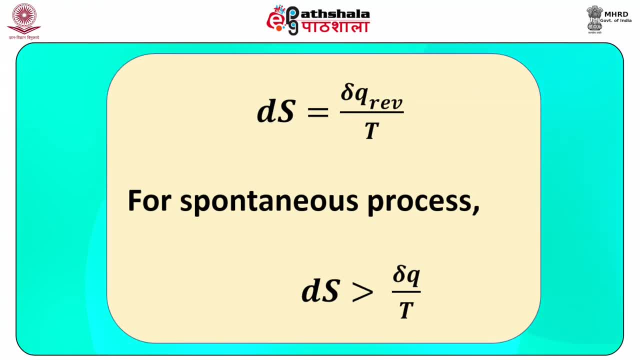 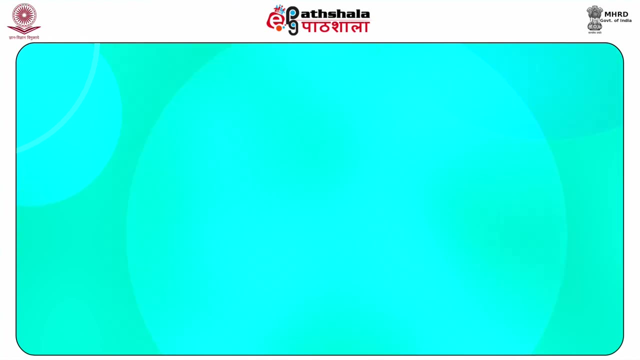 Infinitesimal change in entropy is defined as ds is equal to 0.. For this, ds is equal to del q reversible by t. For spontaneous process, it is defined as ds greater than del q by t. Now we will see the third law of thermodynamics. 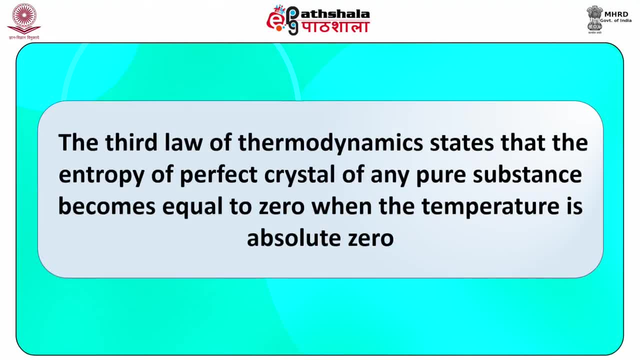 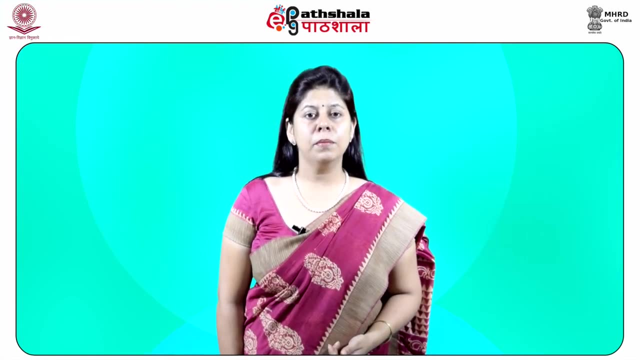 The third law of thermodynamics states that the entropy of a perfect crystal of any pure substance becomes equal to zero when the temperature is absolute zero. At this zero temperature, the system must be in state possessing minimum thermal energy. This system is correct only when the system has one state with minimum energy, Thus at absolute zero temperature. 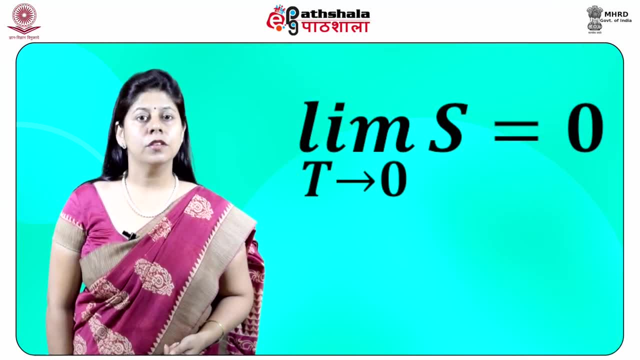 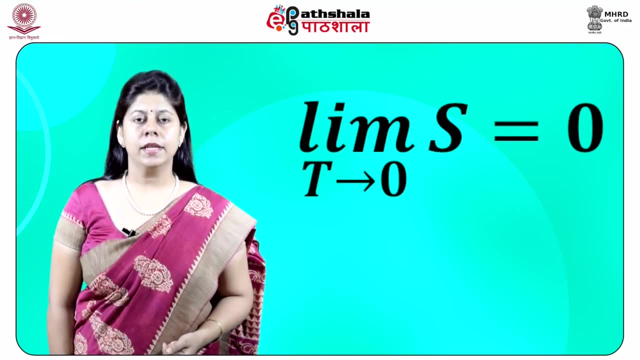 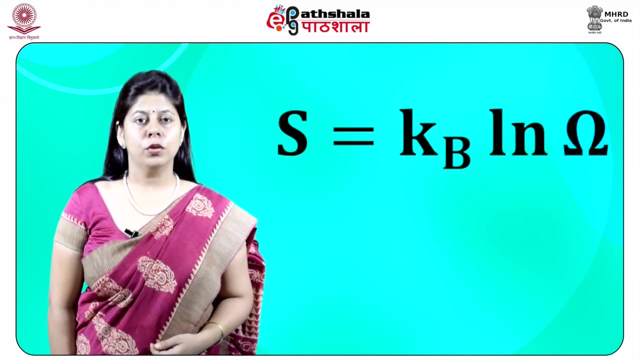 the state is of perfect order, ie zero disorder and hence zero entropy. Therefore, when temperature becomes zero, s is equal to zero. The relation between entropy and and the number of microstates possible for a system is given by. s is equals to kb, ln, omega. 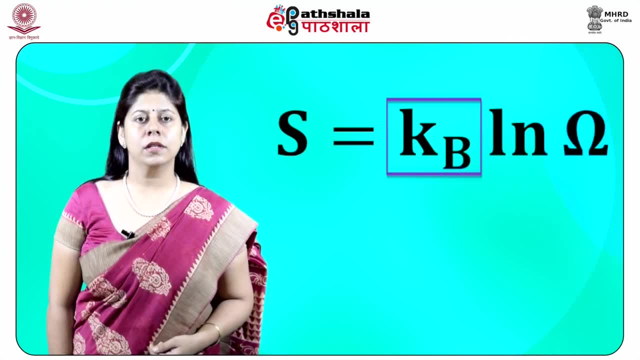 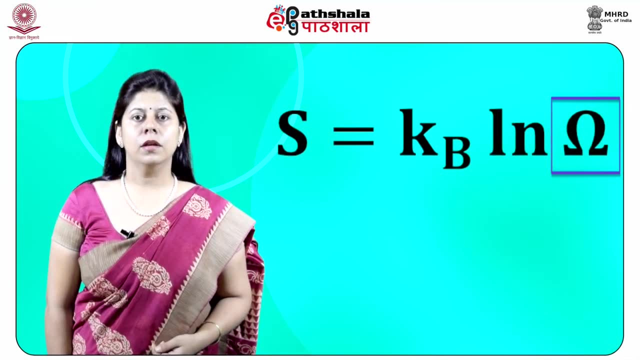 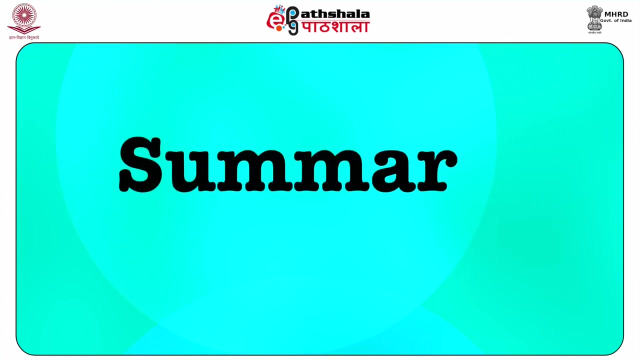 where kb denotes the Boltzmann constant and omega is the thermodynamic probability, which is the number of microstates corresponding the given macrostate of the system. This equation is known as Boltzmann entropy equation. It gives the quantitative definition of entropy as disorder. Now let us summarize what we have learnt. 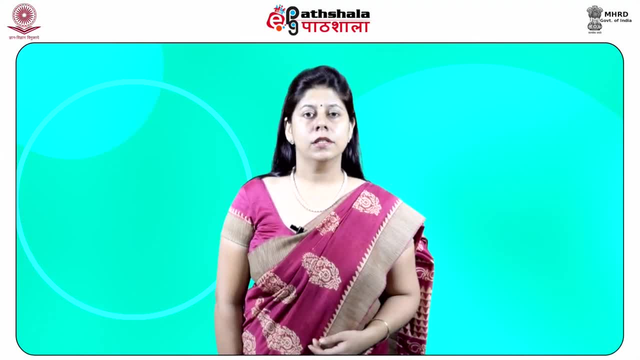 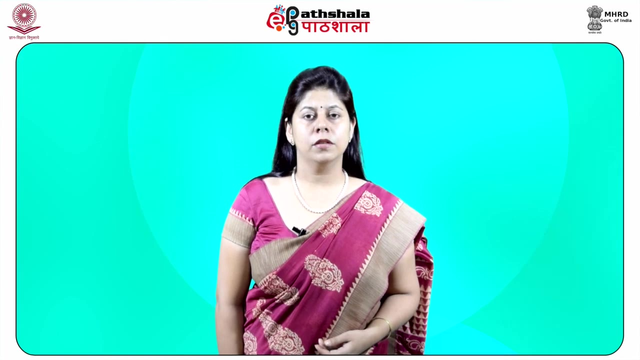 Thermodynamics of irreversible processes essentially deals with the qualitative and quantitative change occurring with respect to time. It is concerned with the transport processes, with the rate of chemical reactions. Equilibrium thermodynamics use the concept of quasi-static process, whereas non-equilibrium thermodynamics use the concept of quasi-static process, whereas non-equilibrium thermodynamics. 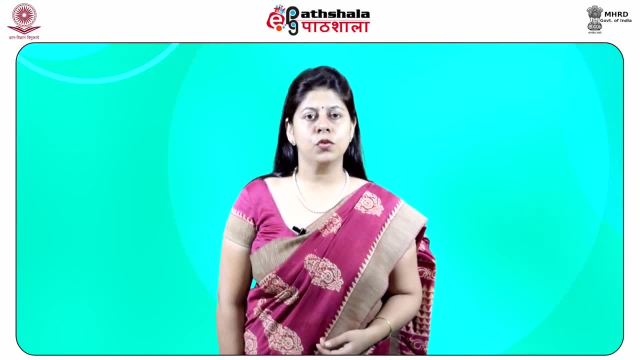 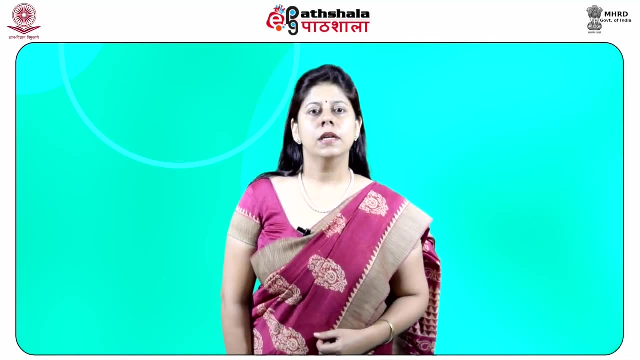 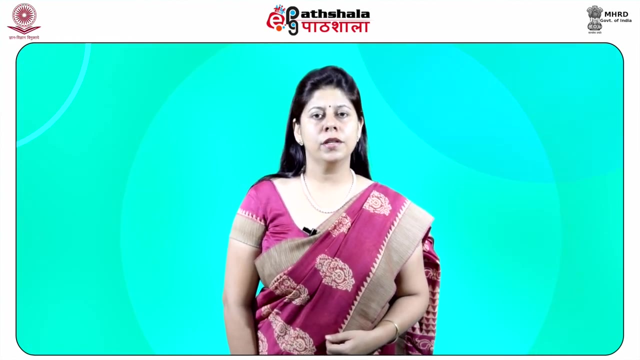 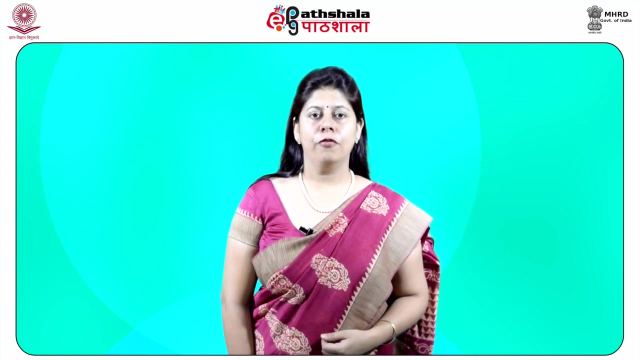 does not use the concept, rather need state variable to describe continuous time courses. Total entropy change of system is the sum of entropy change which arises from its interaction with surroundings and entropy change within the system. The local entropy production sigma is the sum of product of fluxes and conjugate forces. 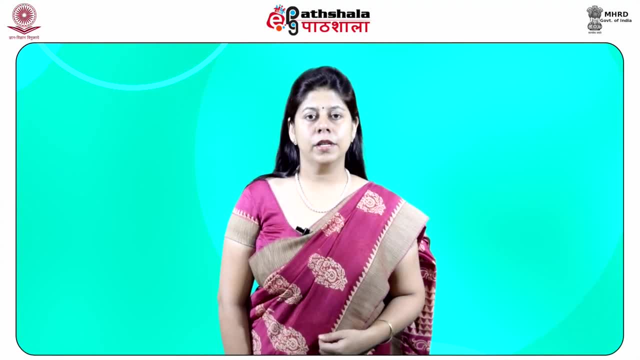 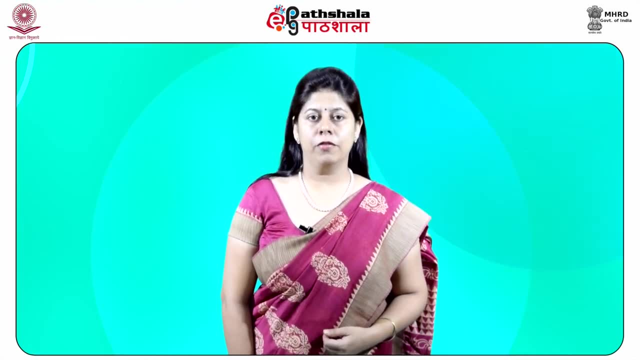 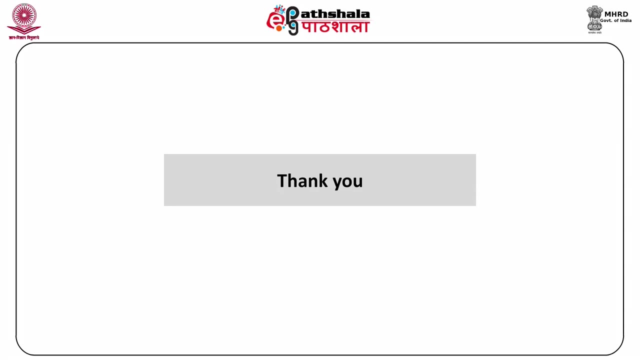 and is therefore given as the total entropy change of the system As the product of Ji into Xi, where Ji is the conjugate force, Xi is the flux and N is the total number of fluxes. We can close the framework of this.